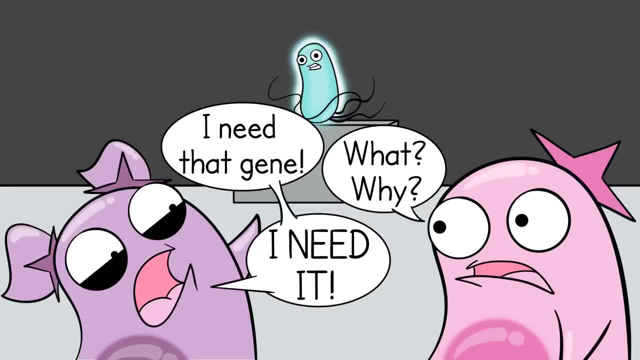 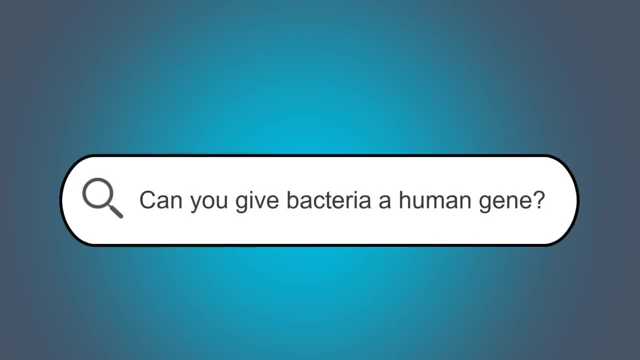 biology courses, but naturally everyone kept wanting to know: is it possible for bacteria to be given a human gene, not just one from a jellyfish? The answer to this class question is yes, And that's when I got to talk about how insulin is produced in the lab. Insulin is 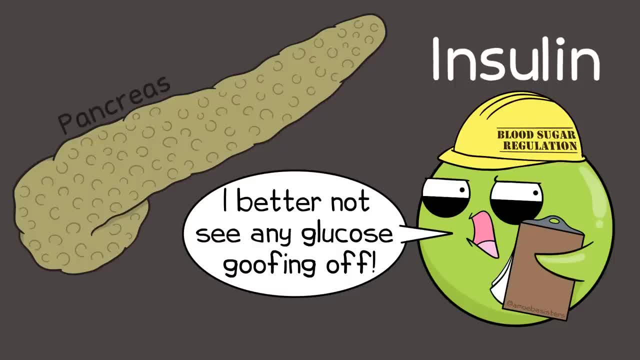 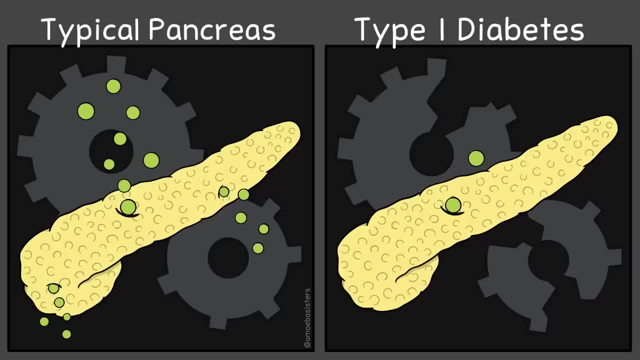 a hormone that all humans need. It is made by the pancreas. The hormone insulin helps make sure that cells get the glucose they need, But type 1 diabetes is a condition where the pancreas doesn't make enough insulin and therefore the individual. 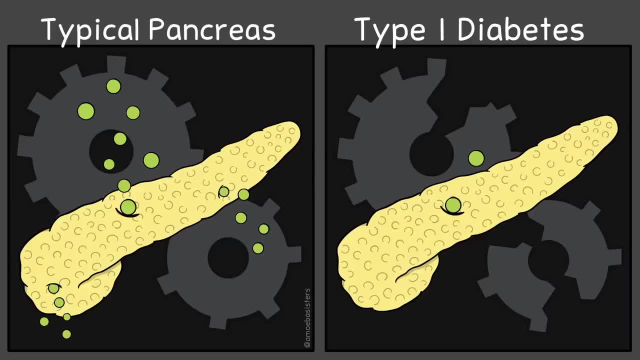 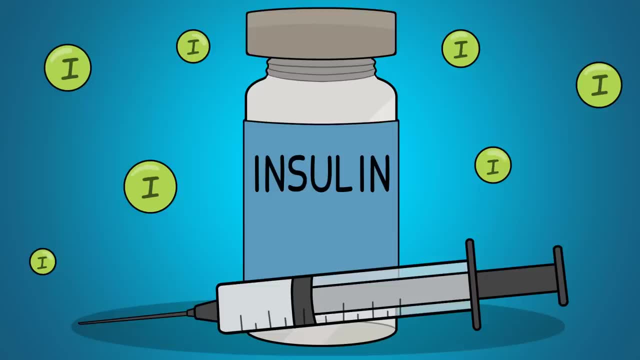 must take insulin, usually in the form of an injection. So how is insulin produced in the lab setting so that those with type 1 diabetes will have an adequate amount of insulin to inject? Well, one current and common way today is by using bacteria in a lab. These 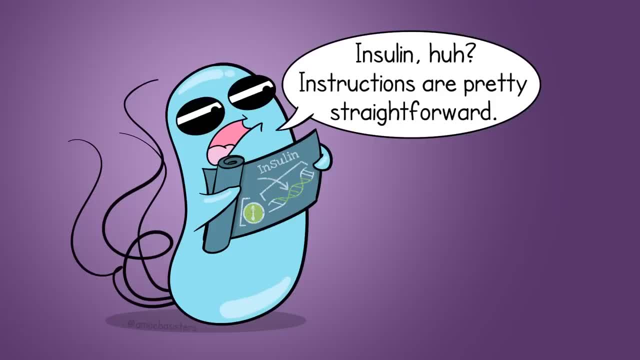 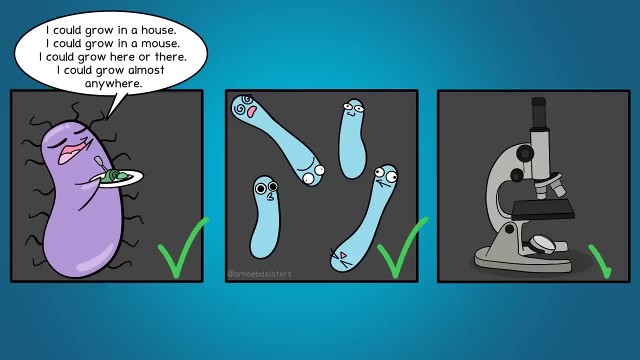 bacteria in a lab can be given the human gene for insulin and then the bacteria produce the insulin. Lots of benefits on that. Bacteria are relatively easy to grow, multiply quickly, don't take up a ton of space. Both the jellyfish and insulin scenarios are examples of transformation, which is the process. 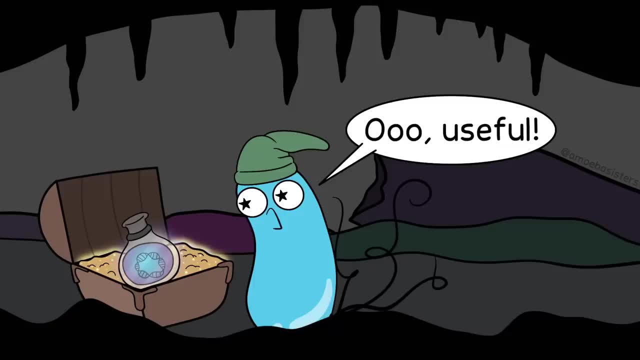 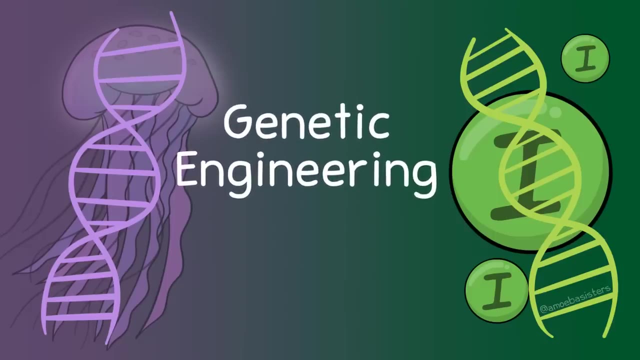 where a cell can take up DNA from their environment and use that. DNA Transformation can occur in nature, but these transformations were specifically performed using genes of interest from other organisms. These two examples fall under the topic of our video: Genetic Engineering. Genetic engineering can be very generally defined as changing an organism's genotype. 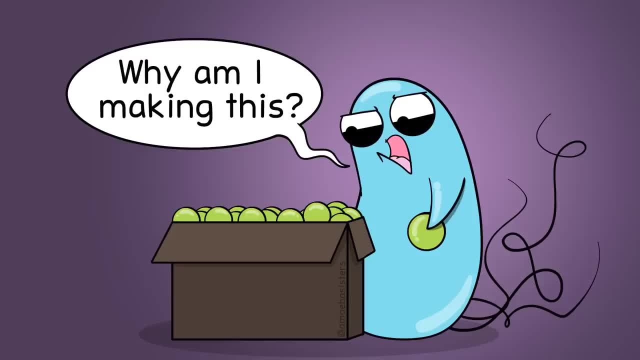 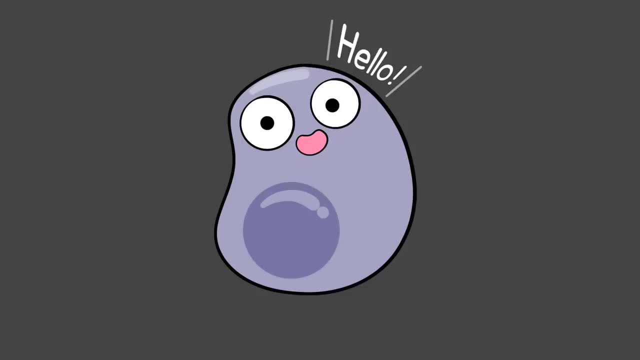 using biotechnology tools or techniques. Let's focus more on the whole bacteria producing insulin example to illustrate how this was done, Focusing first on some basics that we know. Here is a human cell, Like most cells in your body. it contains a nucleus And, like most 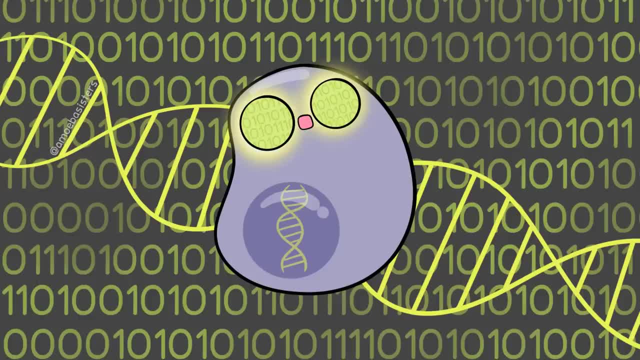 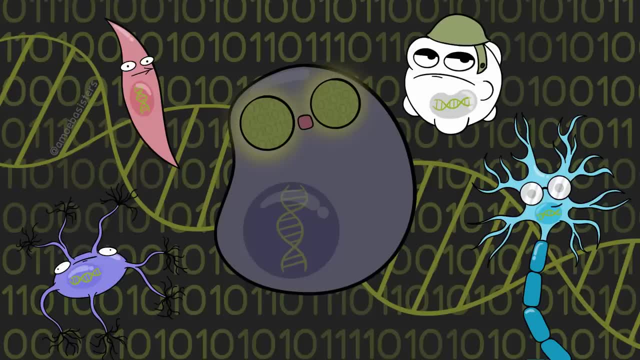 body cells. that nucleus contains the organism's entire DNA code. With some exceptions, each body cell you have contains all of your DNA. If you recall, genes are made of DNA, and so there is a gene that codes for making the protein insulin in most of your body's cells. 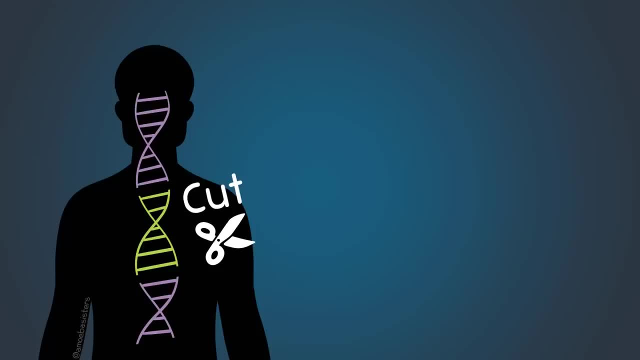 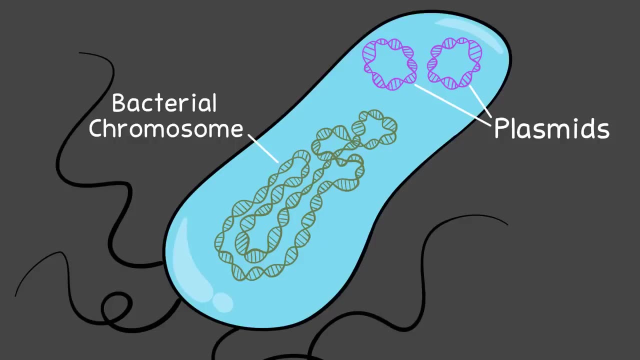 While this gene could be removed from a cell's DNA, the gene for insulin can also be synthesized in a lab. This insulin gene can be inserted into a bacterial plasmid. A plasmid is like an extra set of genes in addition to the bacterial chromosome that bacteria can use. 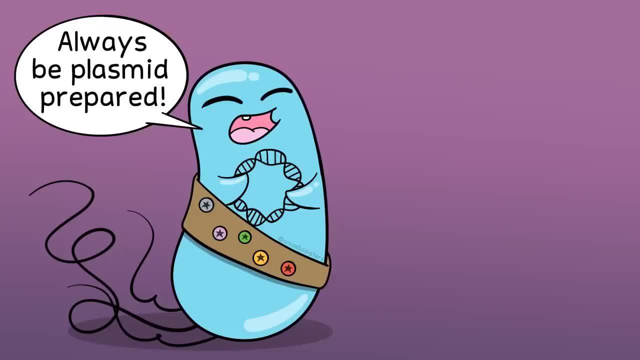 Plasmids tend to be in a circular shape. Plasmids are common in bacteria. You can also find them in yeast cells, But to get specific DNA into the plasmid you have to make sure that you have enough DNA to be able to use it. You can also find them in yeast cells, But to get specific DNA 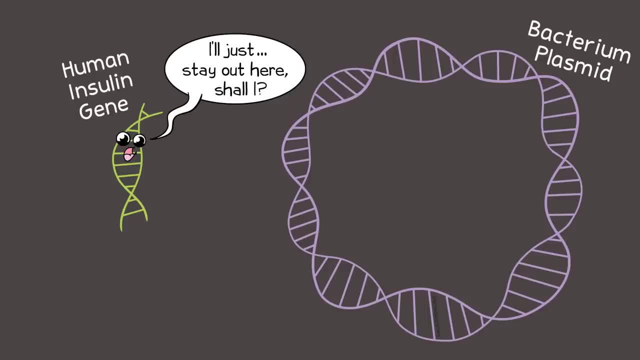 into the plasmid. you have to make sure that you have enough DNA to be able to use it. You have to make space for that. For that you can use restriction enzymes. Restriction enzymes are enzymes that cut in specific spots, like teeny, tiny scissors, and you can cut a specific 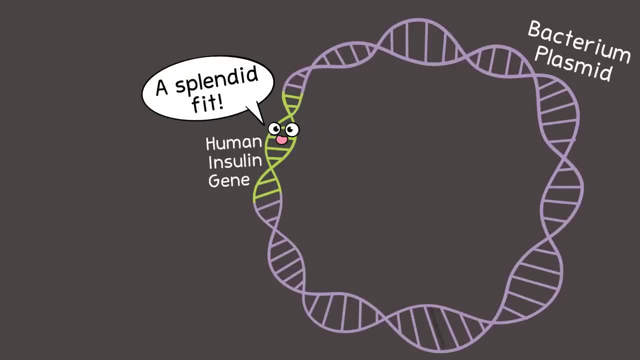 spot in the plasmid so you can add in that human insulin gene Ligase- you remember ligase from our DNA replication video- can be used to help seal it into place. This is now considered recombinant DNA because it contains not only the plasmid DNA but 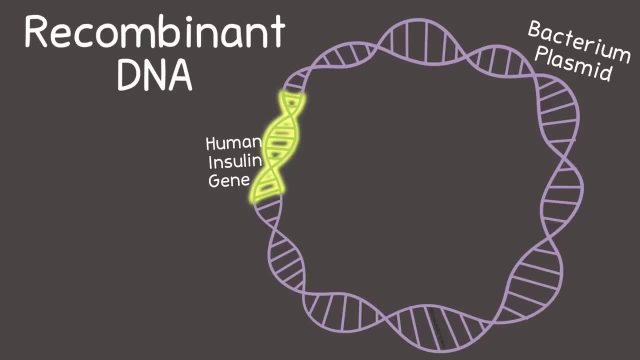 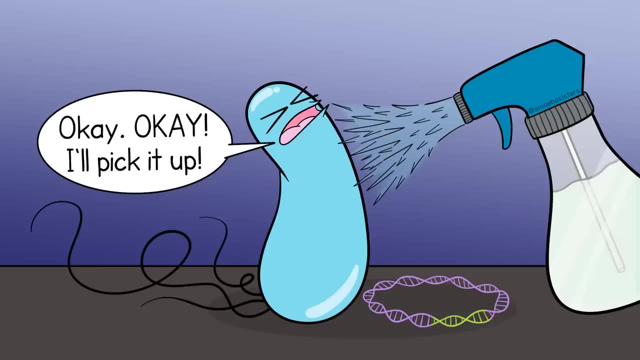 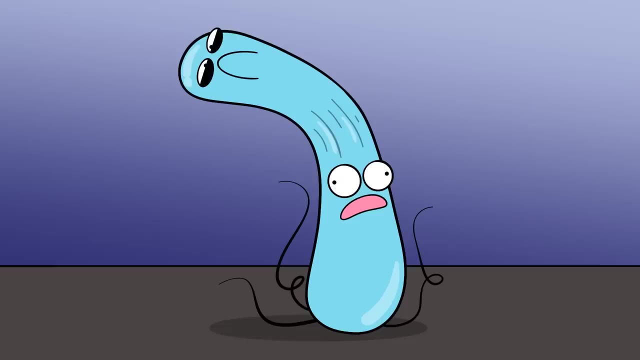 also the DNA of interest, the gene for producing insulin. The recombinant DNA is made up of DNA from different sources. In order to encourage a bacterium to pick up the plasmid in transformation, certain chemicals and temperature changes may be used Once it picks up the plasmid. when the bacterium reproduces by splitting. 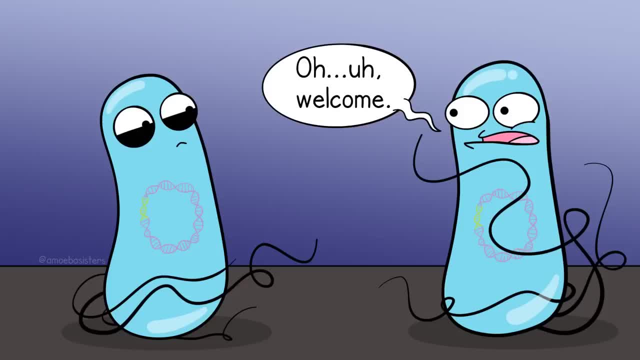 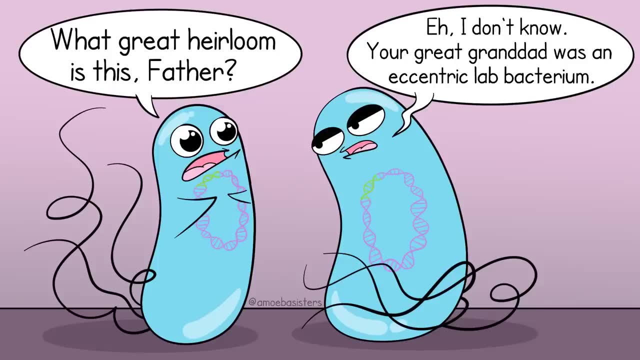 the resulting cells will both inherit the plasmid, And then their daughter cells will inherit it And theirs. You get the picture. In this way, the plasmid continues to be produced over and over. The bacteria can use the human insulin gene to produce human insulin and the insulin can be purified in a lab setting. The bacteria can use the human insulin gene to produce human insulin and the insulin can be purified in a lab setting. The bacteria can use the human insulin gene to produce human insulin and the insulin can be purified. 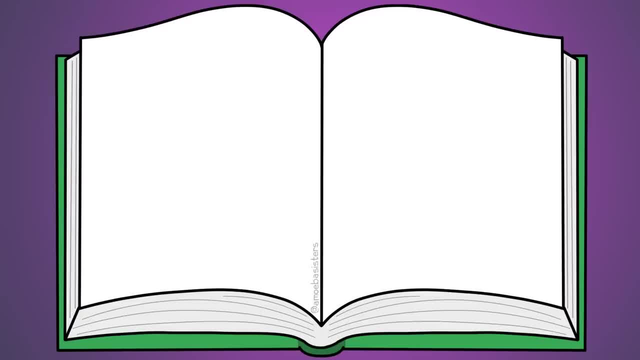 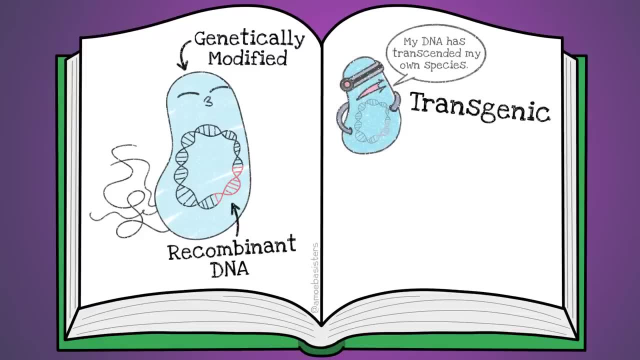 in a lab setting to be used for humans. Let's talk about some vocab in our example. In this example of genetic engineering, the bacteria were genetically modified from recombinant DNA. You can consider the bacteria to be transgenic. Any organism or microorganism that has genetic material from some other organism is considered. 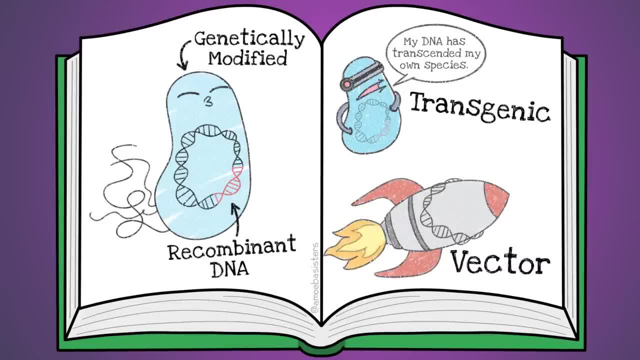 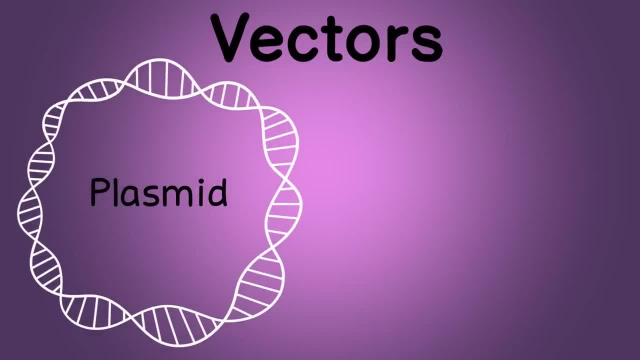 transgenic. The plasmid was the vector in the situation. A vector can be thought of as a vehicle for getting the recombinant DNA into the organism. Plasmids are a common vector, But plasmids aren't the only vectors in genetic engineering. Viruses are another example. 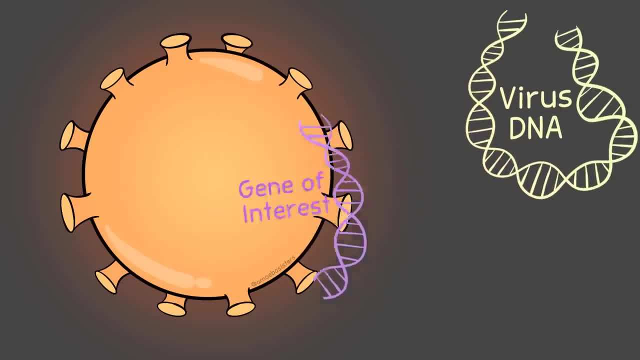 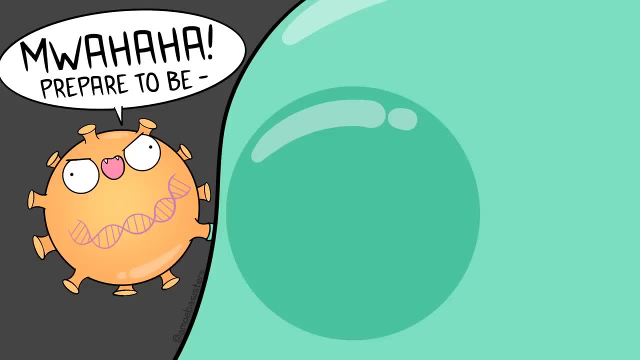 If a virus's own genetic material is removed and a gene of interest instead is placed inside, the virus can then be permitted to attach to target cells to deliver that gene of interest. When it attaches to a target cell, it inserts the gene of interest Viruses in this way. 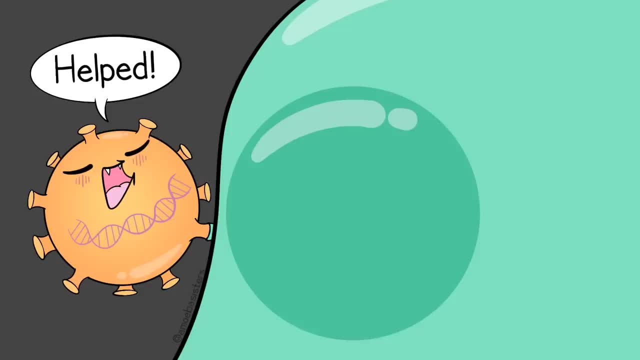 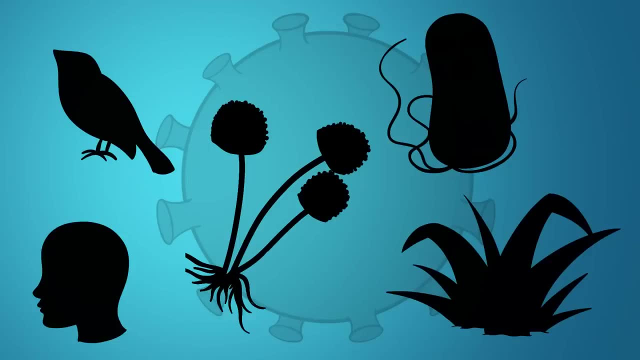 are another delivery system, And viruses can target any kind of living cell: Bacteria, fungi, plants, animals, including humans. You can find examples of viruses in our description, Sometimes, if the plasmid or viral vector is just not ideal for delivering DNA into. 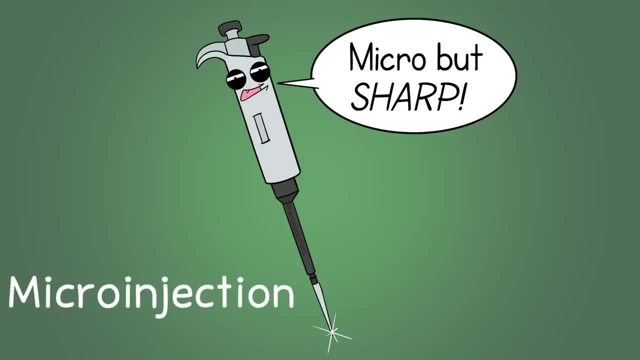 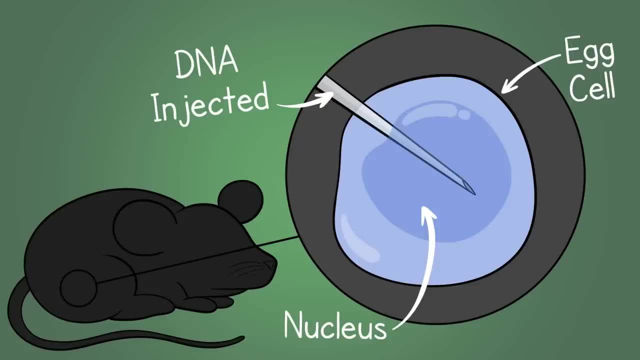 a cell. well, you have more options. There's microinjection. A special kind of micropipette can inject the gene of interest through the cytoplasm of a cell and into the nucleus, For example, if the target was a fertilized mouse egg cell. Or- and I didn't learn about, 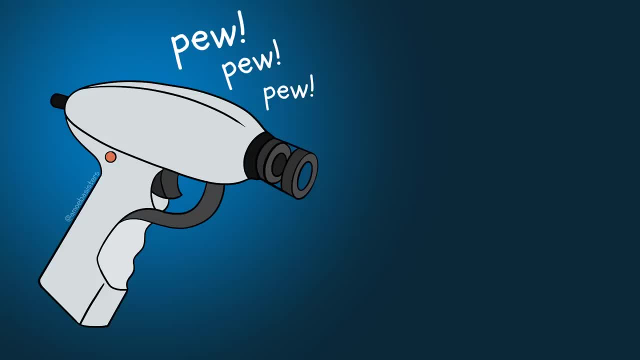 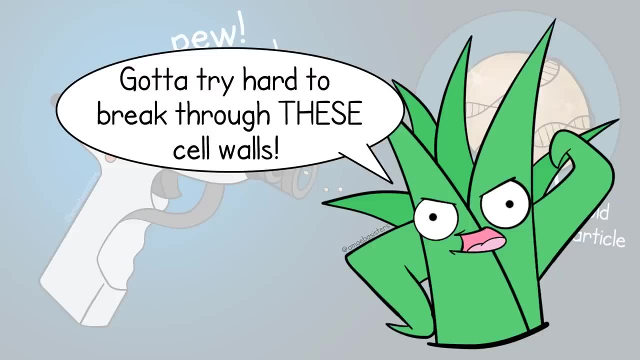 this until more recently. gene guns- Yes, really, a gene gun can shoot particles- gold particles, for example, that are coated with DNA- Really helpful in cases where you have thick cell walls to get through, like a plant cell. Genetic engineering techniques and tools continue to develop and change. 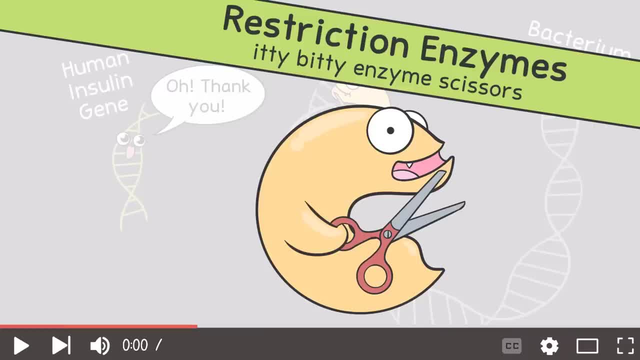 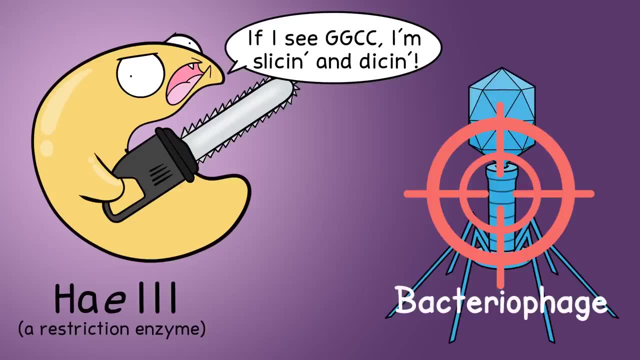 So when we were talking about restriction enzymes and we mentioned they cut in specific spots. they have certain sites that they recognize And anytime that site exists they cut. Restriction enzymes are actually part of the natural defense system bacteria have against bacteriophages. 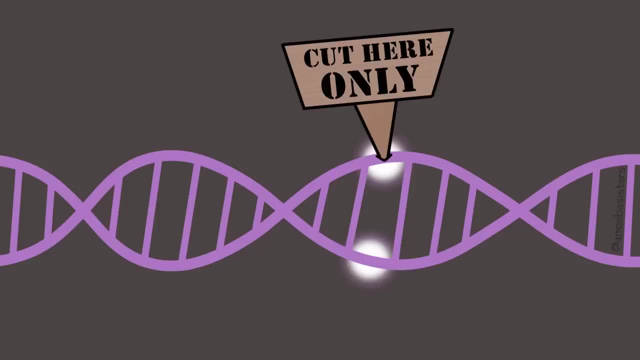 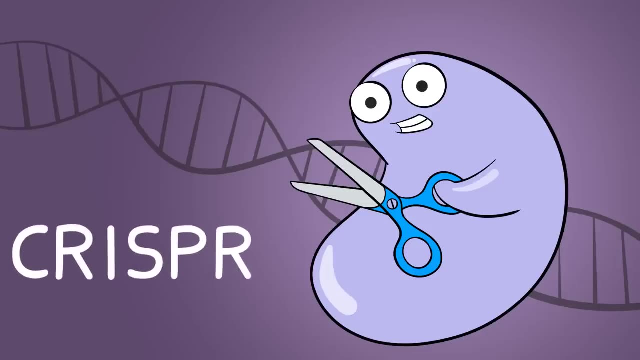 They can chop up bacteriophage DNA, But what if you had a way to customize the exact place you want to cut in the DNA? Perhaps you've heard about CRISPR. This gene editing tool allows for the editing of DNA using a special kind of. 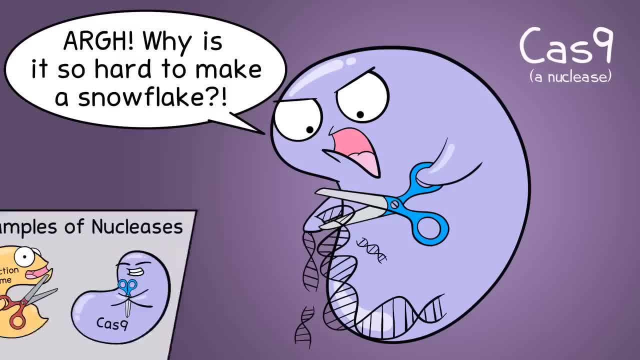 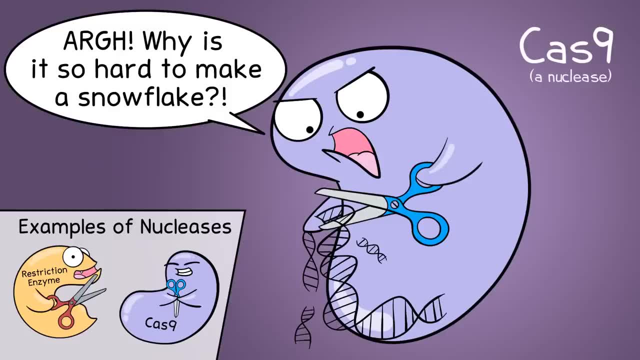 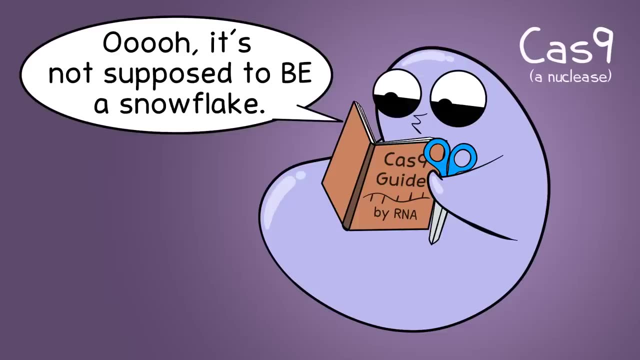 nuclease called Cas9. Recall that nucleases like restriction enzymes and Cas9, can cut DNA And like restriction enzymes, the CRISPR-Cas9 system is also part of the natural defense system bacteria have against bacteriophages, But in CRISPR by using a specific guide, RNA. 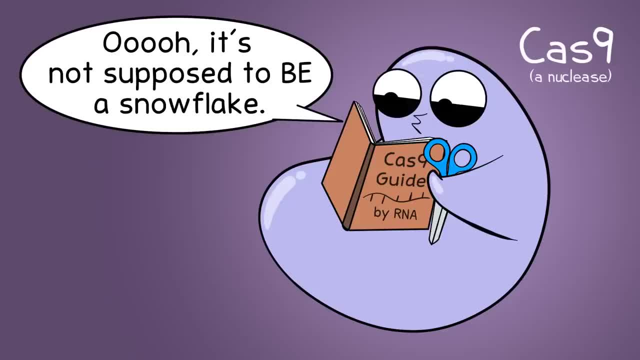 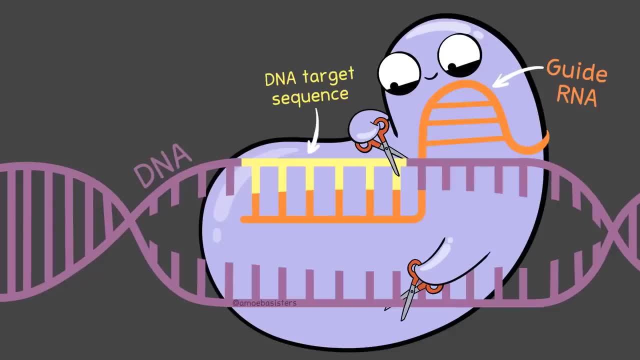 that can be designed in the lab. the Cas9 can be guided with the specific guide RNA to cut it points around a specific target gene And by doing that one can do gene editing by removing a selected target gene And, if desired, a new gene could be inserted in its. 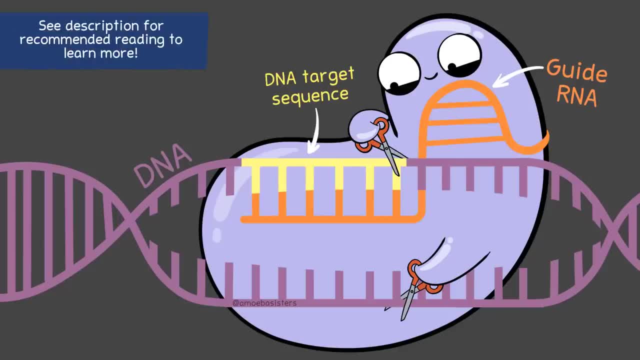 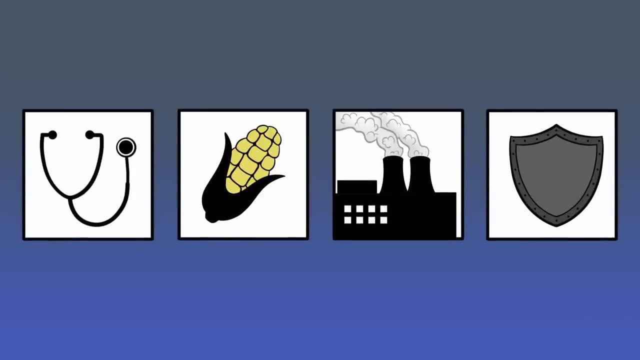 place. CRISPR has been used in plants and animals, including clinical trials of humans. So now that we've covered some ways that genetic engineering can be done, we want to address how can genetic engineering be useful? There are tons and tons of examples of uses.